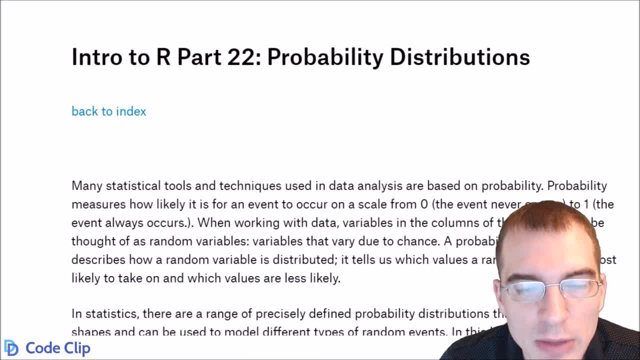 Hello everyone and welcome to Introduction to R, Part 22,: Probability Distributions. So in this lesson we're going to discuss what probability distributions are and how to work with them in the R programming language. So many statistical tools and techniques used in data. 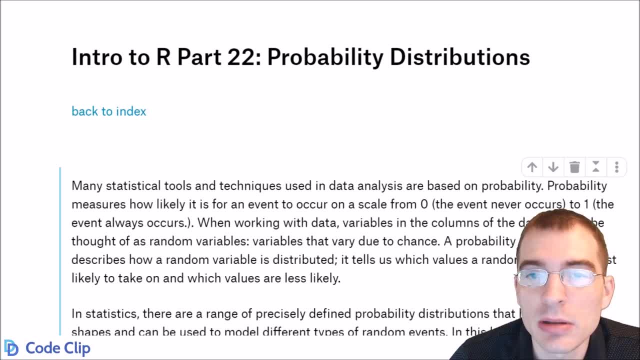 analysis and machine learning are based on probability, and probability is just a measurement of the likelihood that some event is going to occur. that is on a scale from zero, which means an event never occurs, to one, which means the event always occurs. In working with data, the 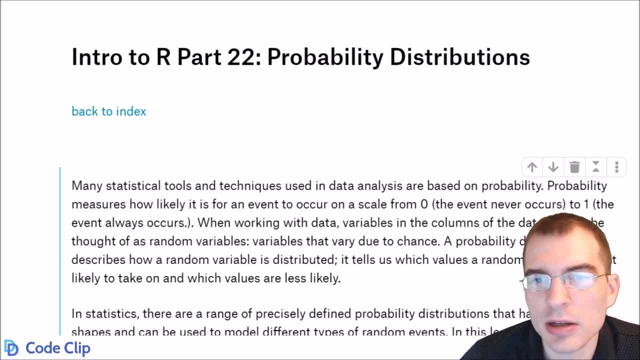 variables you have in the columns can be thought of as random variables, which are variables that vary due to chance, And a probability distribution tells us which values a random variable can take on And also which values are more likely than others. Now, in the real world, we don't have access to the 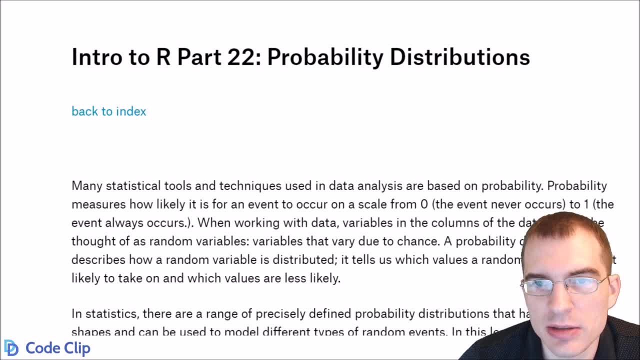 actual probability distributions that generate the data that we see. We don't really completely understand processes that generate data, so we use approximations to model what the underlying probability distributions might be, And there are many different, precisely mathematically defined probability distributions in statistics that have different shapes and different properties that 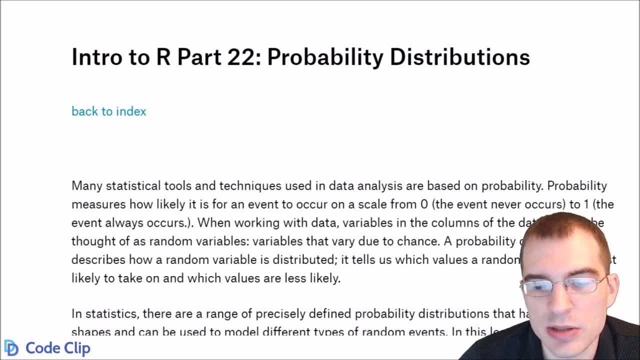 can be used to model different sorts of random events. So in this lesson we're going to discuss what some of those well-defined probability distributions are and how to work with them in the R programming language. So I'll start by looking at the uniform distribution to learn the 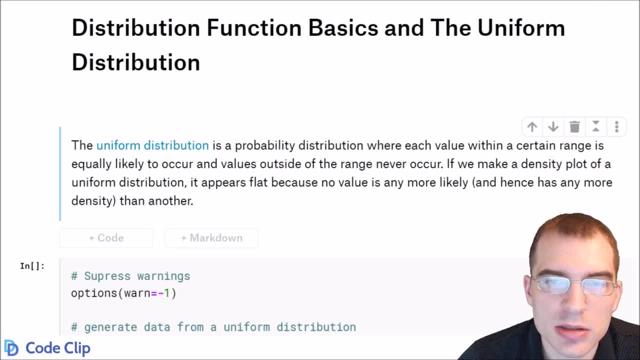 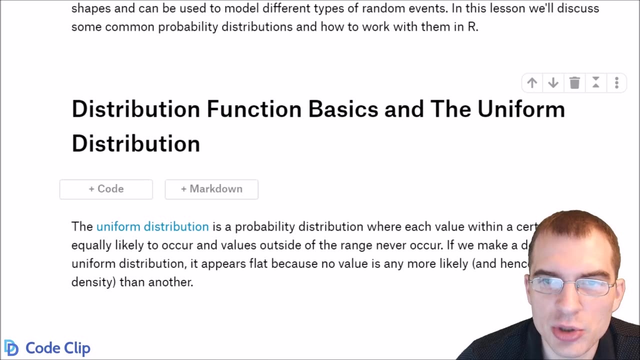 basics of probability distributions in R. So the uniform distribution is just a probability distribution where every single value is equally likely to occur. So I'll just start by generating a bunch of numbers using a uniform distribution and plotting it so we can see what a uniform 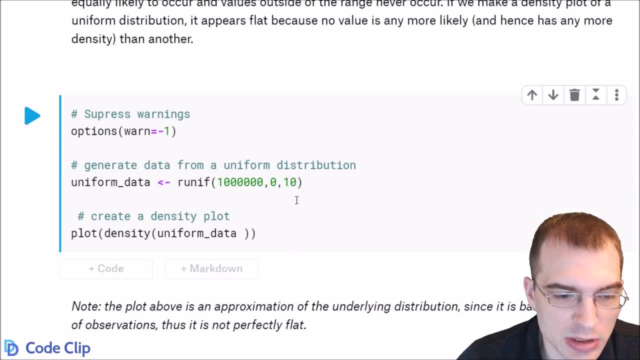 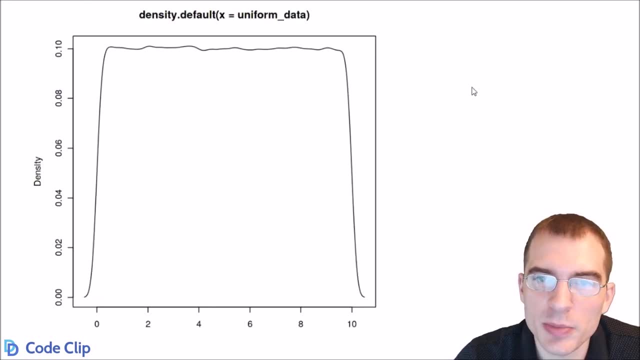 distribution looks like. So we're just going to generate a bunch of uniform data and plot it. It's going to be on the range from 0 to 10.. So this is a density plot of the uniform data that we generated. Now, a probability density function is just a plot. 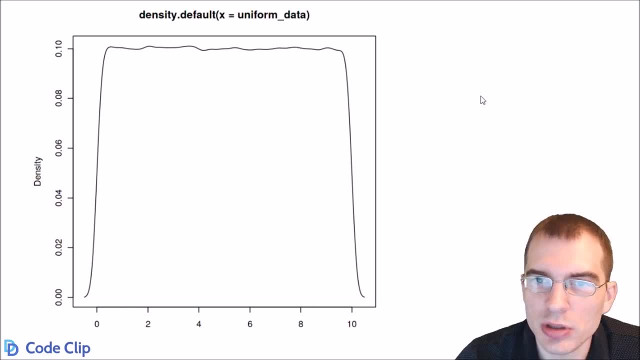 It's a plot that shows the distribution of a random variable. It's a graphical representation of where certain values are more likely and other values are less likely. In this case we are generating random data uniformly from 0 to 10.. So the density of a uniform distribution. 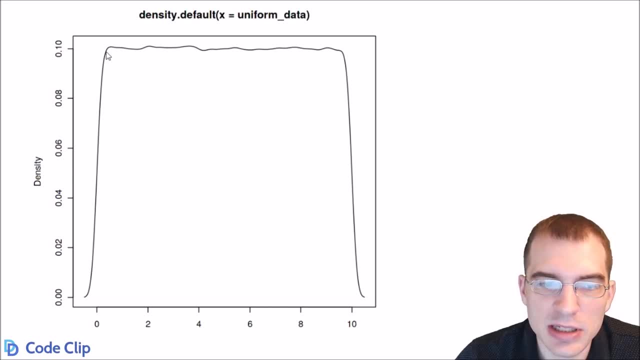 is flat because everything is equally likely. You can see, our plot is actually not completely flat. It's a little bit wiggly because we actually generated this data randomly, So there is a little bit of natural variance in here. that didn't make it completely flat, But what this means is every single value we could have generated. 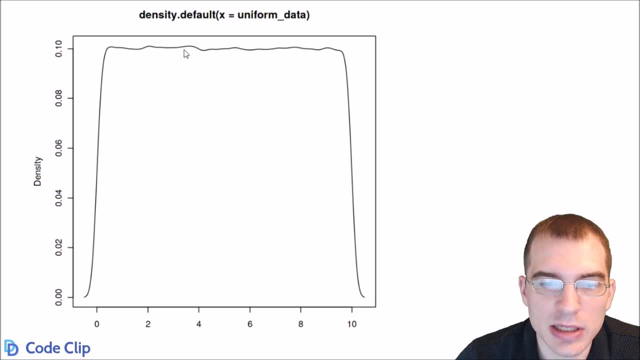 from this range was equally likely to be selected. That's why it's pretty much just a flat distribution, And it should be noted that the volume or area under a probability curve like this always sums up to 1.. So, since we generated from 0 to 10 and the density is 0.1 and it's 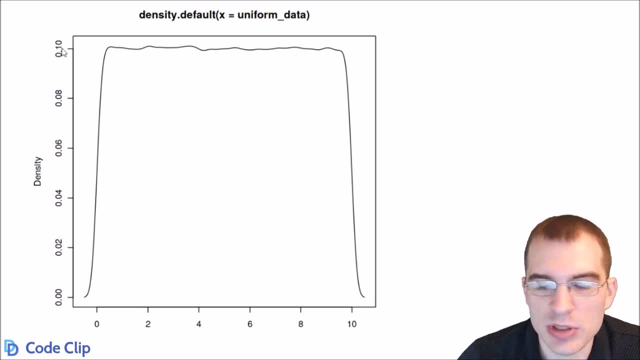 constant. if we multiply those together, which essentially amounts to integrating this, because it's just a square distribution- would sum to 1.. In general, if you check the area under a probability density curve, no matter what type of density function it is, it always has to sum to 1.. 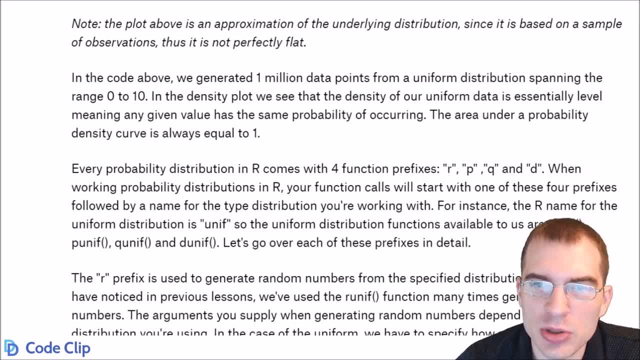 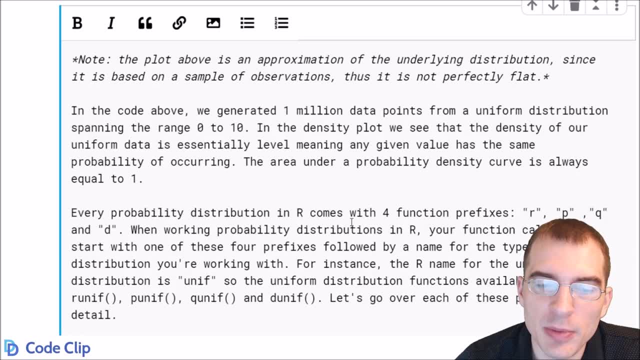 Now every probability distribution in R comes with a special shorthand name to use to work with it. In the case of the uniform distribution it's UNIF, And probability functions also have four different prefixes. you can use to work with them in R. 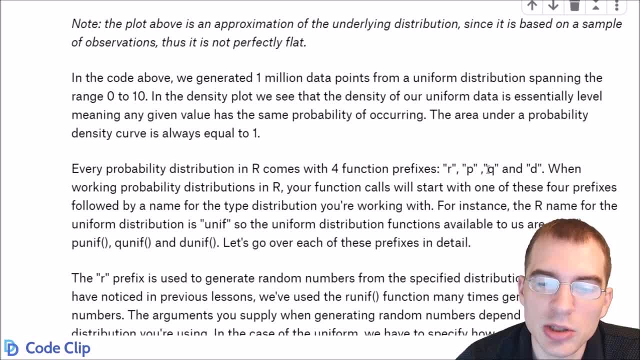 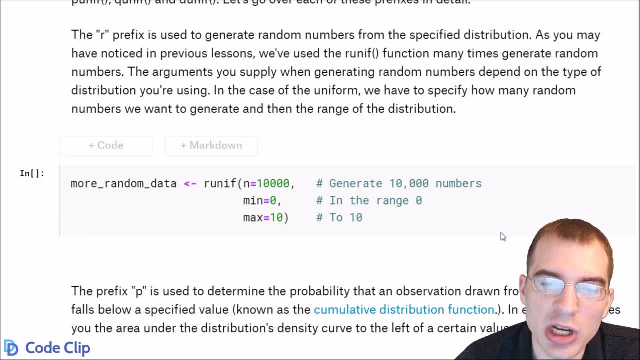 They are the R prefix, P, Q and D, So I'll spend a bit of time going into what each of those means. The R prefix is what's used to generate random numbers from the specified distribution. So above, when we generated all the numbers we used to make that plot, we used the R UNIF function. 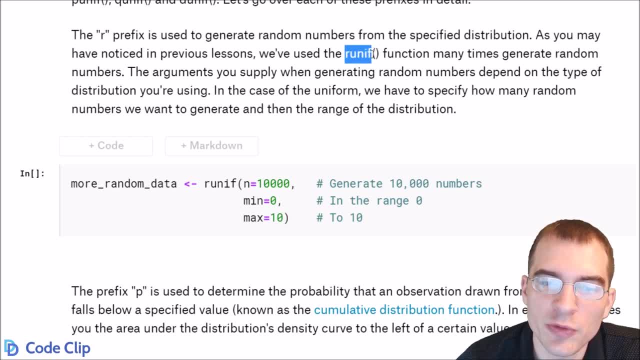 that means we're generating random numbers from the uniform distribution. So we'll see another example of how to do that here. We're going to generate some more random data. We're using R UNIF. That means generate random numbers with a uniform distribution. 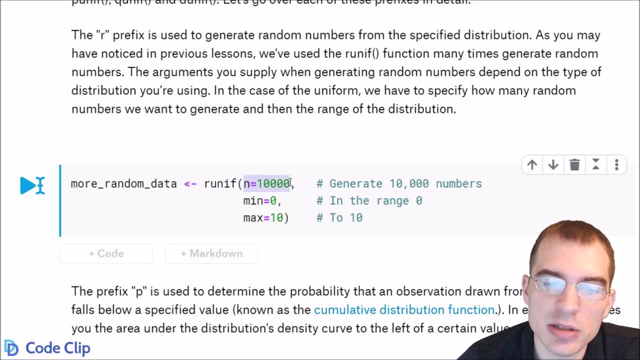 N is the first argument, which is how many numbers you want to generate. Then you just have to enter the min and max, which is the range of the uniform distribution. So here we're generating 10,000 more random values between 0 and 10.. And now the P prefix is used to. 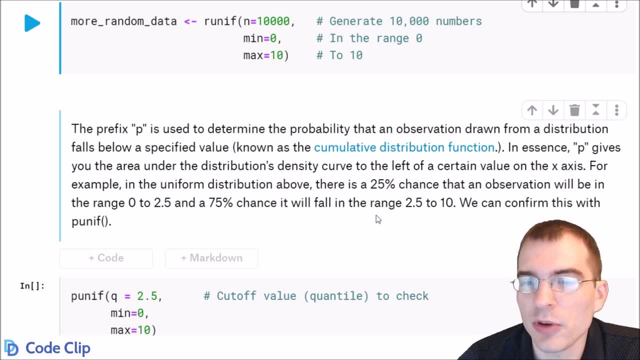 determine the probability that an observation drawn from a distribution falls below a specified value. This is also known as the cumulative distribution function. So, in essence, P gives you the area under the distribution's density curve, that's to the left of a certain value along the x-axis. For example, in the uniform distribution we made above, 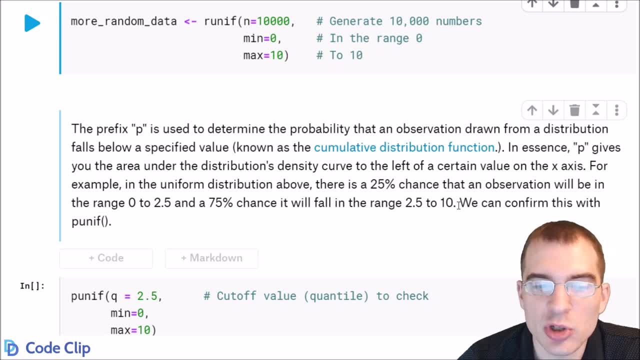 there's a 25% chance that an observation will be in the range between 0 and 2.5, and a 75% chance that it would fall between 2.5 and 10.. And we could confirm this exactly by using the P UNIF function. Let's do that. We're going to run P. 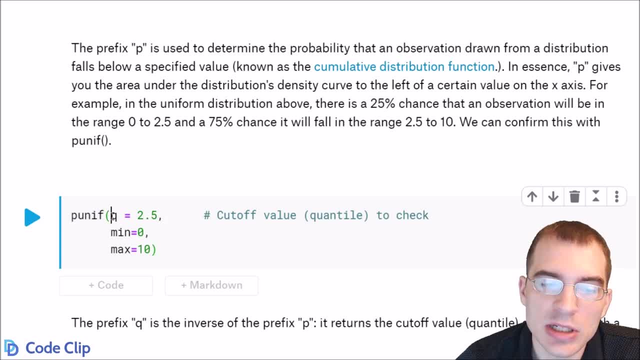 UNIF. The first argument is Q, which is the quantile or cutoff value that you're checking at. In this case, we wanted to check at a cutoff of 2.5.. And since we're checking for the same uniform distribution, we're going to again enter a min of 0 and a max of 10.. 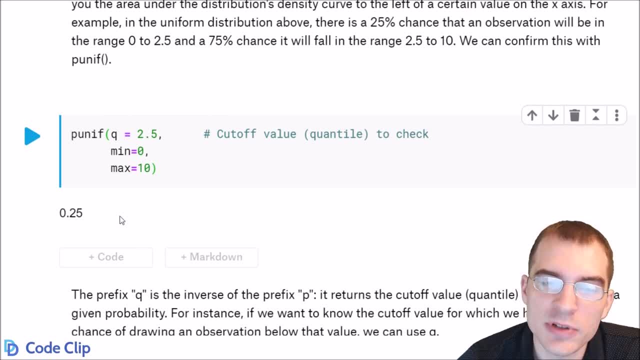 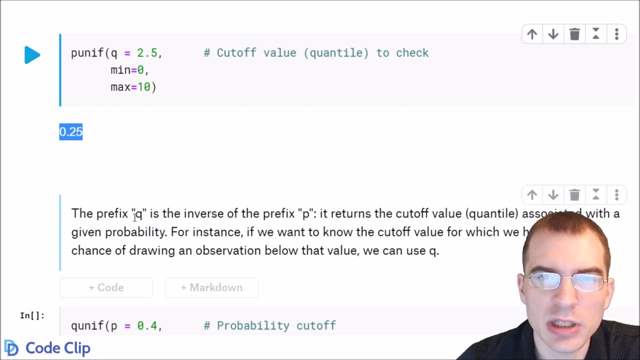 When we run that as expected, the area to the left of 2.5 under this uniform distribution curve is 0.25, which means we would have a 25% chance of having a number generated in that range. The Q prefix when working with probability functions in R. 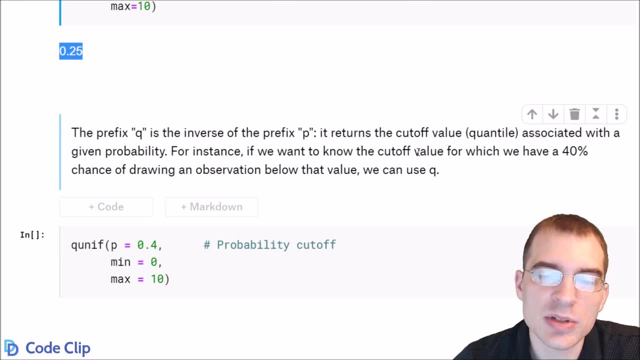 is kind of the inverse of P. It returns the cutoff value or quantile associated with a given probability. For instance, if we wanted to know the cutoff value for which we had a 40% chance of drawing an observation below that value, we could use q. So we'll show. 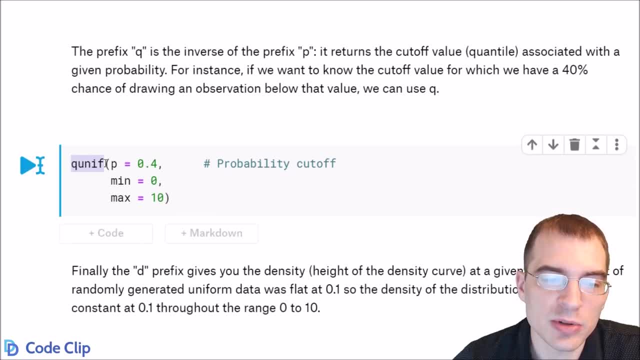 an example of using that, We're going to use qunif, which means we're checking the quantile of the uniform distribution. In this case we wanted to check a probability of 40%. So the first argument is that probability p is 0.4.. Again, we're going to use the same range for 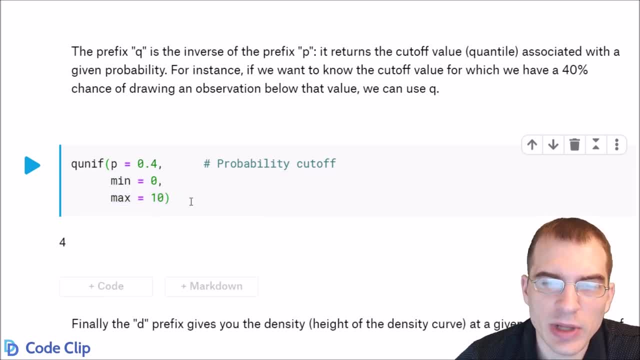 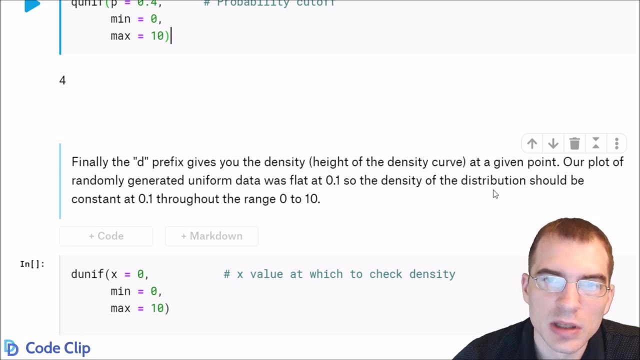 the distribution, So as we can see the quantile that we would have to set to cut off the first 40% of observations, in this case is 4.. And finally, the d prefix gives you the density or height of the density curve at any given point. Now, if you recall, in the density curve we 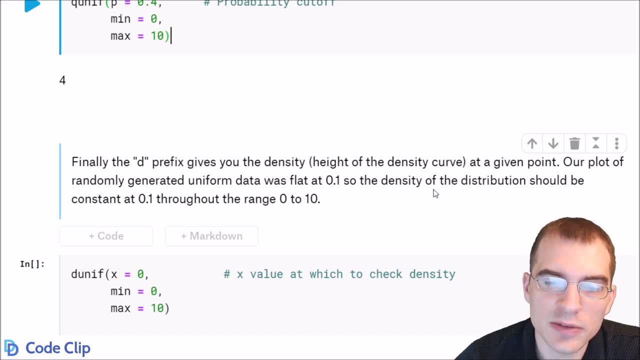 generated, the data was flat with a height of 0.1.. So that means the density given by the d prefix on that distribution should be 0.1,, regardless of where in the range we check. So we'll use the dunif function. 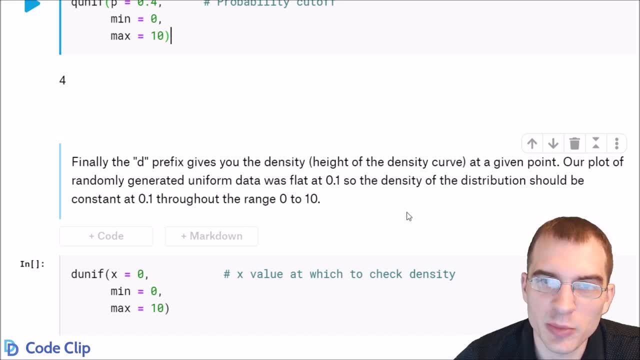 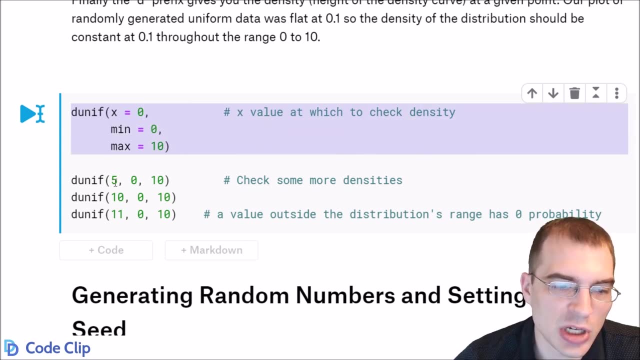 And we'll check that, And we'll check a few different points just to confirm that it's going to be the same everywhere. And we're going to check x equals 0.. We're also going to check x equals 5 and x equals 10.. All of those should be 0.1, because it's just flat And it doesn't. 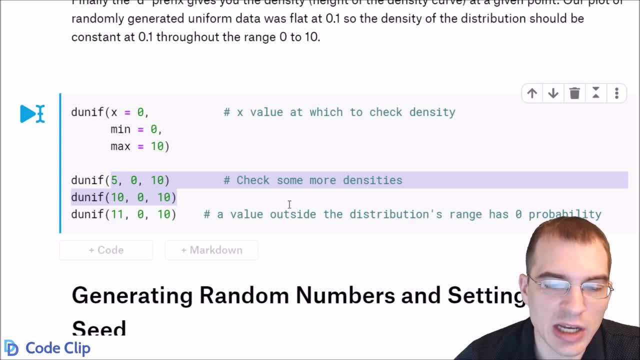 change throughout that range. But if we try to check a value outside of the distribution's range, it's going to show up as 0, because the chances that there's an 11, it's impossible because the range of the distribution only goes from 0.1.. So we're going to check that And we'll check. 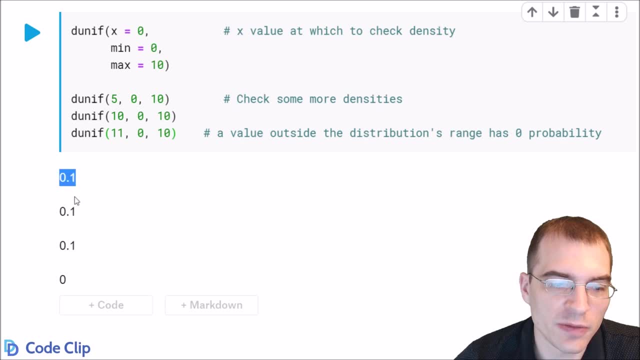 x equals 5 and x equals 10.. So we'll run that And we can see we did get 0.1 for all the ones that were within the range. Anything outside of the range is going to be 0.. So before we start talking, 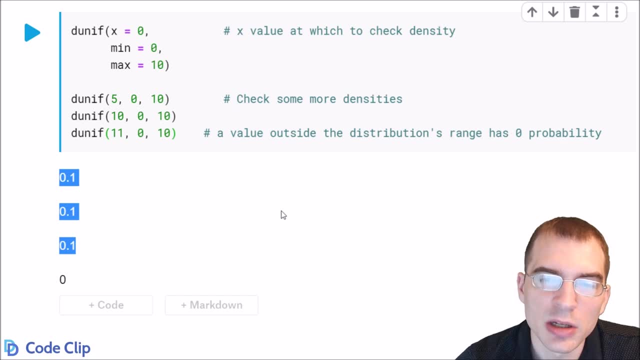 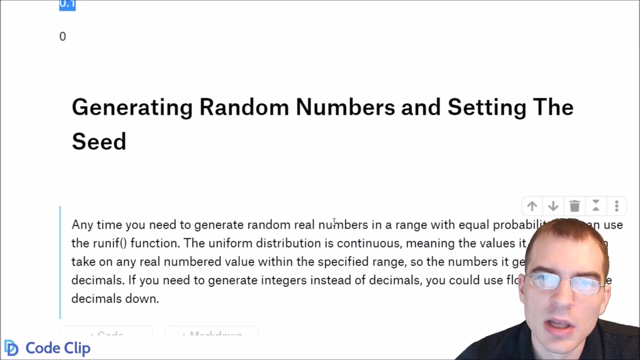 about other probability distributions and how to work with them in R. we're going to have a quick aside and talk about generating random numbers and setting the random seed. So anytime you need to generate random numbers of equal likelihood in R, you can use that Runif function that we 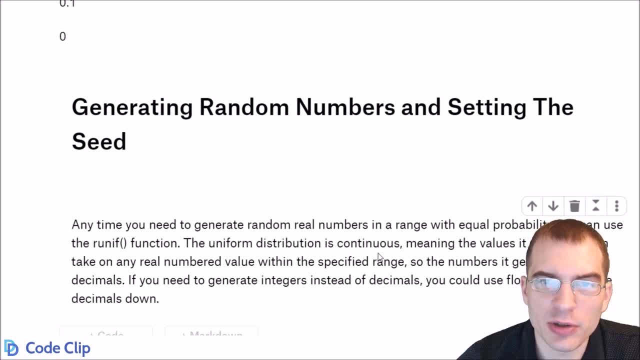 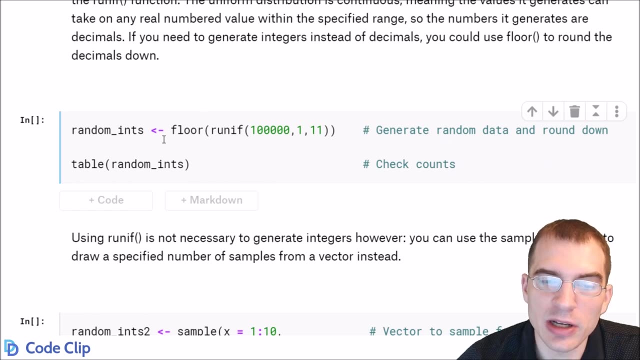 looked at earlier, And this will generate real numbered or floating point value numbers within a specified range. If you wanted to not have decimal numbers and just have integers, you could do that just by rounding, whatever the generated numbers are. So, for instance, if we wanted to get random integers, 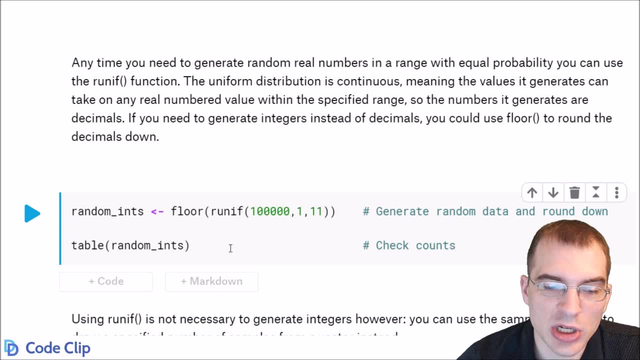 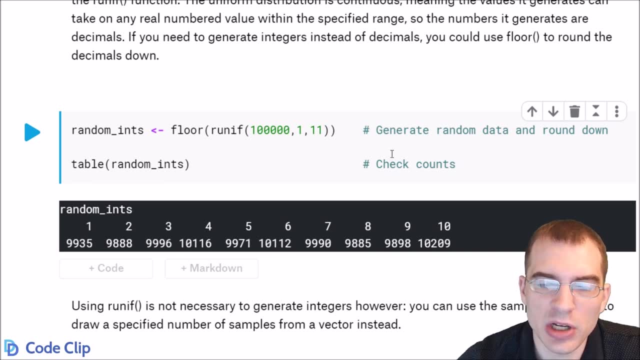 we could use the floor function, So just run this and check a table. They should be mostly the same, but of course there's some randomness involved And this is a little bit of a roundabout way of generating integers. You can actually do this easier using the sample function, So I'll show how to do that here. 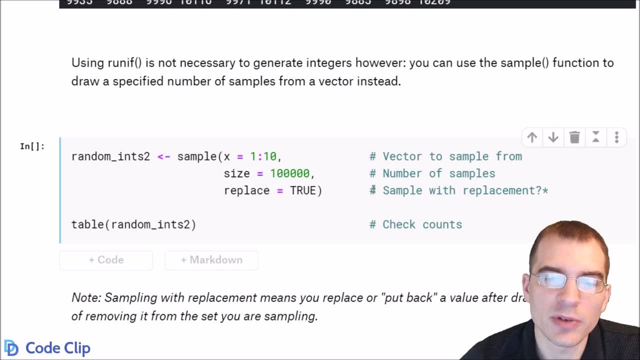 With sample. you just pass in a range of, or vector of, values you want to generate randomly from. In this case, we're going to generate numbers between 1 and 10, but we could pass any vector in here. Then the second argument is size, which is the number that you want to sample. 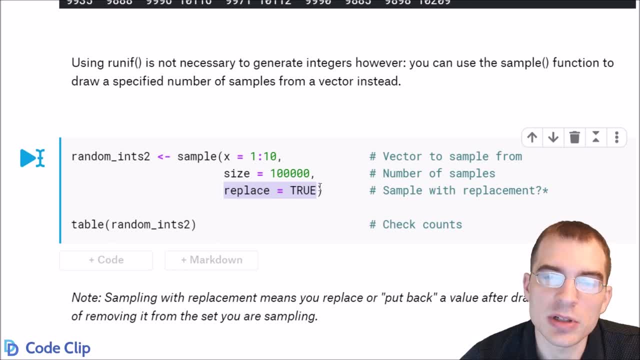 And replace is whether you want to sample with replacement or not. We want to be able to generate values more than once, So we're going to say, well, I'm going to do this, And then we're going to say sample with replacement. But if you put false, you're essentially taking any value you draw. 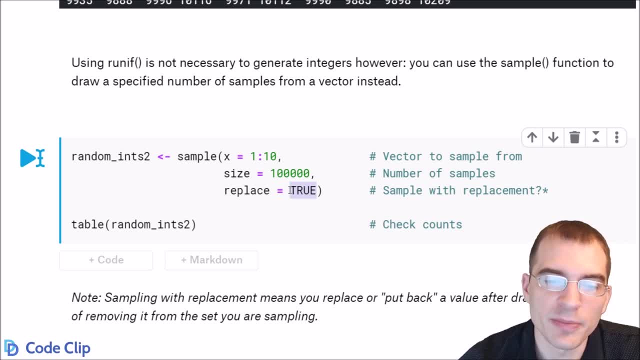 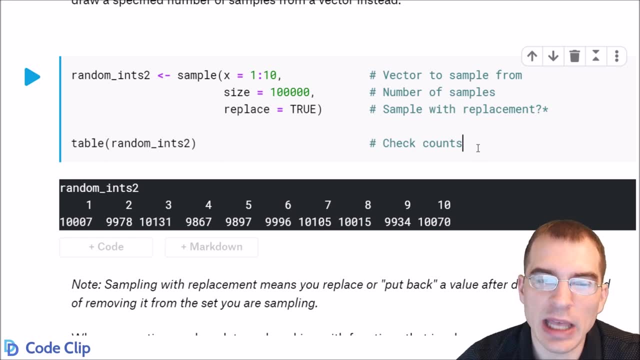 is not returned back into the pool of values you're drawing out of. So if we run this, it will essentially do the same thing as above, but a little bit nicer. So it's important to keep in mind when you're doing anything in a programming language. this isn't specific to R, but programming. 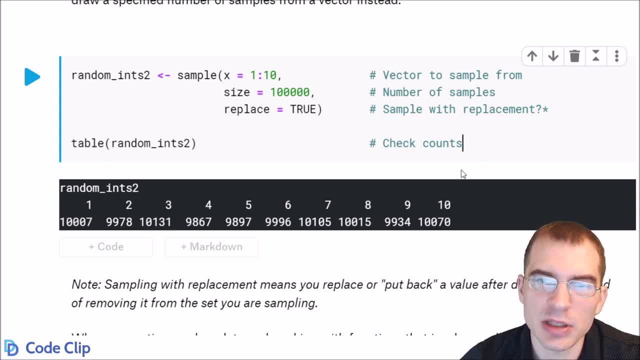 on computers in general, whenever you're doing something that involves randomness, you're generally dealing with what's known as pseudo-randomness. So there's a random number generator that is generating numbers with some complicated formula, but computers are ultimately deterministic machines. So if the random number generator 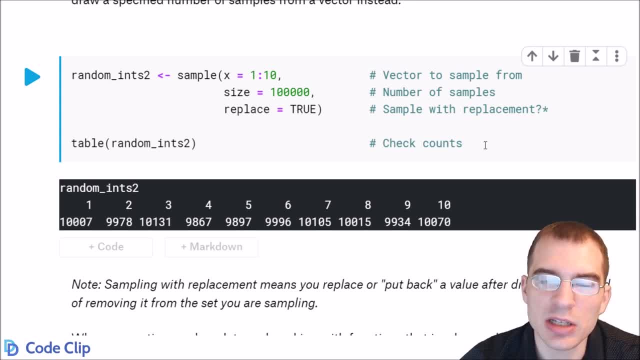 is initialized to the same initial state, you're going to get the exact same outcome for random numbers that you generate. So numbers generated by computers are not truly random, unless you can actually sample some form of true randomness. So if you, for instance, had some kind of sensor that was able to sample some source of true 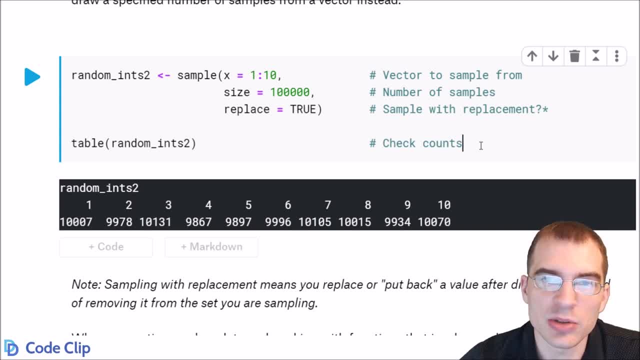 environmental randomness, then you could use that to get true random numbers. But anything that's being programmatically generated is not truly random, And this is not necessarily a bad thing, because it means you can precisely reproduce anything you do, even if it involves randomness. 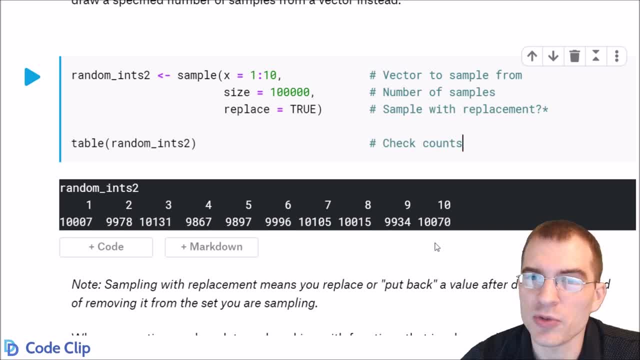 But if you want to, you can do that by using a random number generator. So if you have a random number generator and you want to reproduce something that involves randomness, exactly you need to store the value that was used to initialize the random number generator. 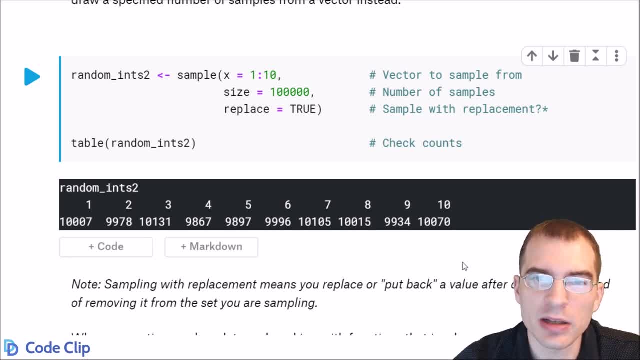 So if you want to do that, you need to do what's known as setting the random seed, and that will initialize the random number generator to a given state before you run something And every time you rerun it if you set the same seed. the functions that involve: 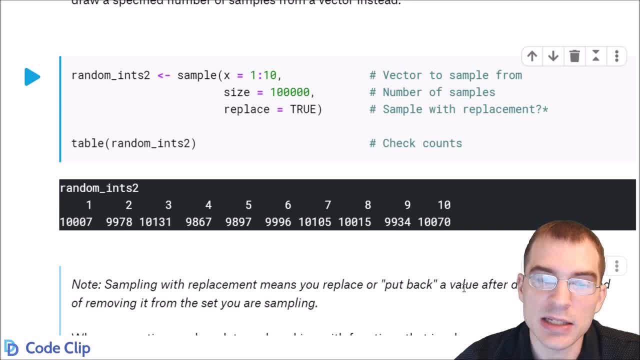 randomness that you're using will actually produce the exact same results, So we'll just show how to do that. In other words, if you want to reproduce something that involves randomness, you need to set the random number generator to a given state before you run something that involves randomness. But if you don't want that, that's okay, All right, Some people took a couple of minutes to do that, so I'll give you a couple more minutes to do the same thing. So here, what I'm just going to do is just set the random seed to zero and then I'm just going to give it an arbitrary nothing, and 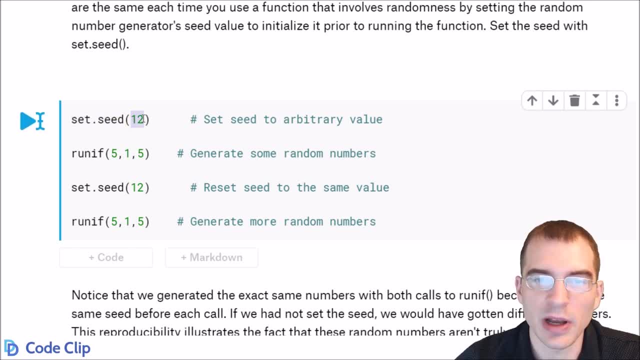 then I'm just going to pass in an arbitrary value into that function And you'll get different results depending on which number you pass in here. But as long as you use the same one every time, the results will be the same. So we're going to generate these numbers twice and we'll 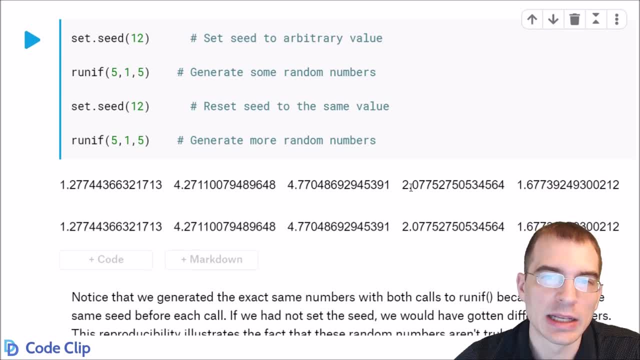 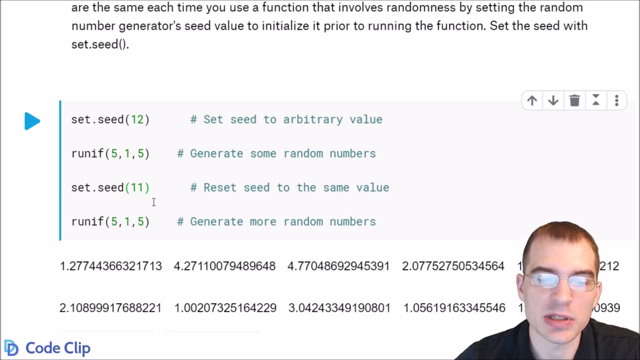 get the same numbers, even though they're supposed to be random. Now, if we went back and, for instance, change this initial seed to something else and we ran it again, then the numbers would not be the same. So whenever you want to do reproducible data science and you're using 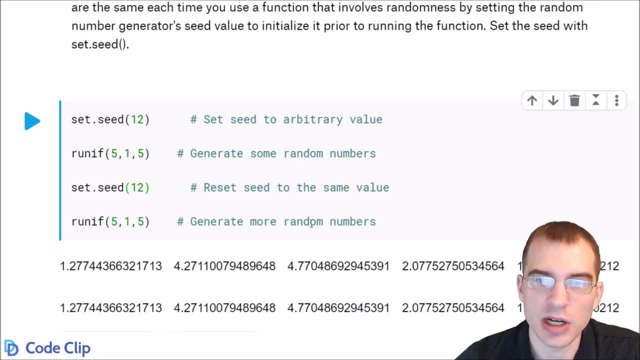 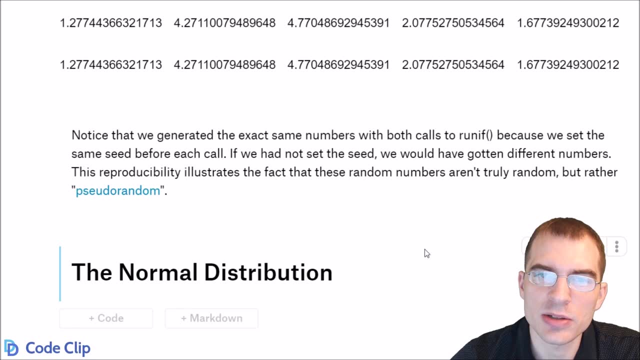 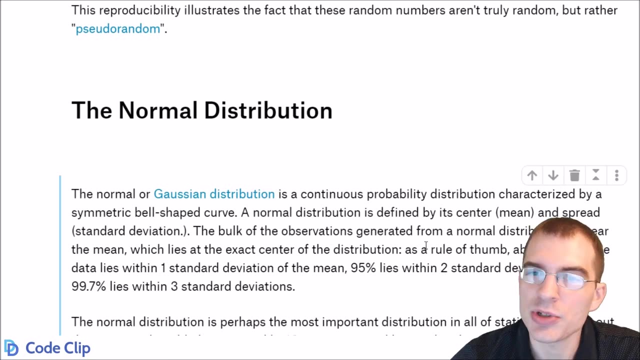 randomness, then you can use this setseed to accomplish that. So now I'll continue just by going over some of the different common probability distributions that you're likely to want to deal with in R and data science in general. We'll start with the normal distribution, or Gaussian. 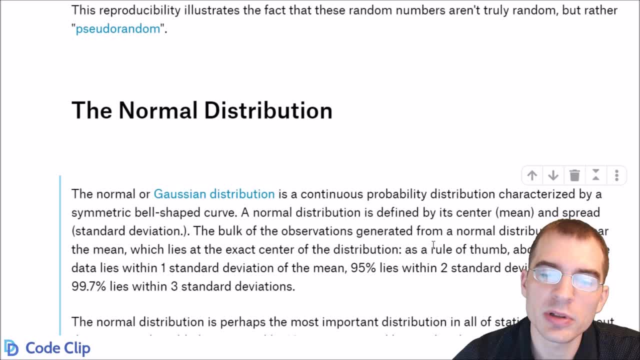 distribution. Now, this is a continuous probability distribution characterized by a bell-shaped curve. continuous just means it can take on any value within a given range, including decimal values, whereas a discrete probability distribution only takes on a fixed set of values. For instance, a coin flip would be an example of perhaps the most simple probability distribution you could. 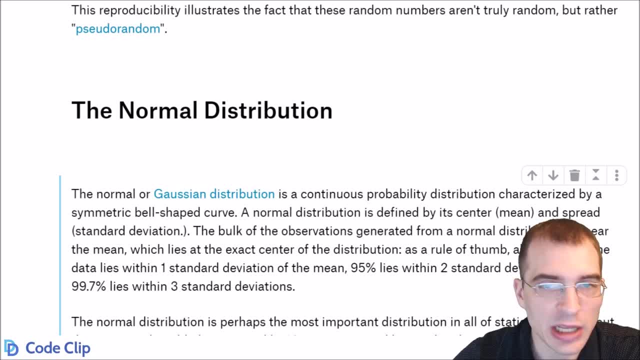 think of, and it only takes on two values, either heads or tails, which you could say are like getting a zero or a one. In fact, in statistics there's a special name for a certain value for this type of distribution. that is essentially a coin flip that can only take on one of two values. 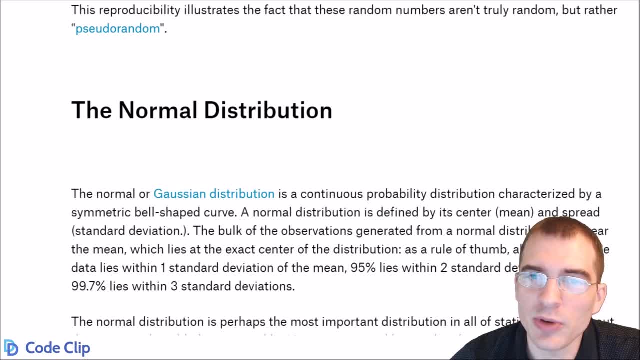 with some probability. It is known as a Bernoulli random variable. The one caveat is: with a coin you're generally thinking that it's a 50-50 coin flip probability, whereas with a Bernoulli distribution there's a parameter p which determines the likelihood of getting a success or not. So 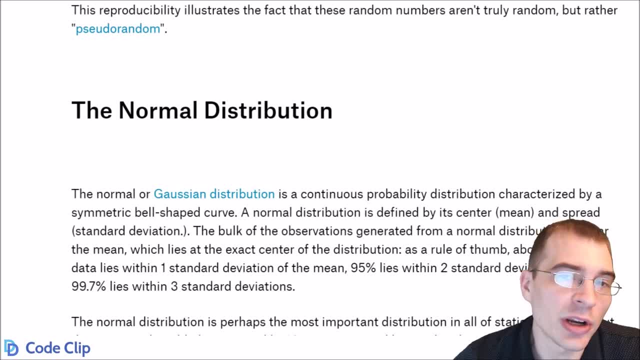 with the Bernoulli random variable. you might have an unfair coin where you might have a probability of, say, 80% of getting a one, or you could say that's like a heads and a probability of only 20% of getting the other value. But back to the normal distribution. 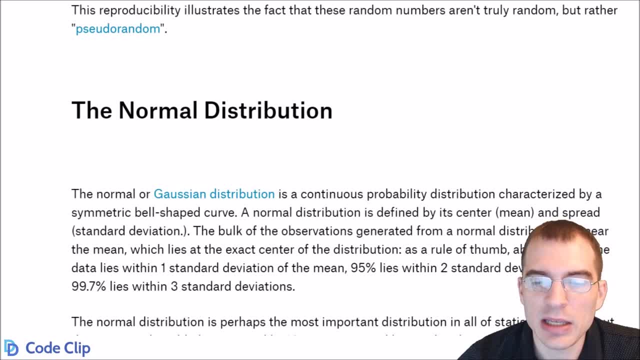 it is a continuous distribution which is defined by its center, which is the mean or average, and its spread, which is its standard deviation. Now, the bulk of the normal distribution is centered around the mean. As a rule of thumb, approximately sixty-eight percent of two has the same count. 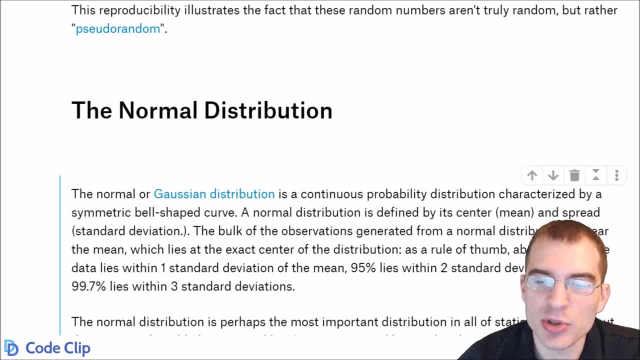 whereas the bulk of the normal distribution is centered around the mean. as a rule of thumb, 0.68% of a normal distribution's data is within one standard deviation of the mean, 95% lies within two standard deviations and about 99.7% lies within three standard deviations. So when people 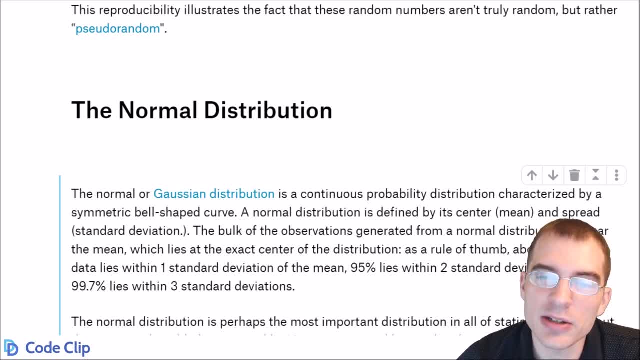 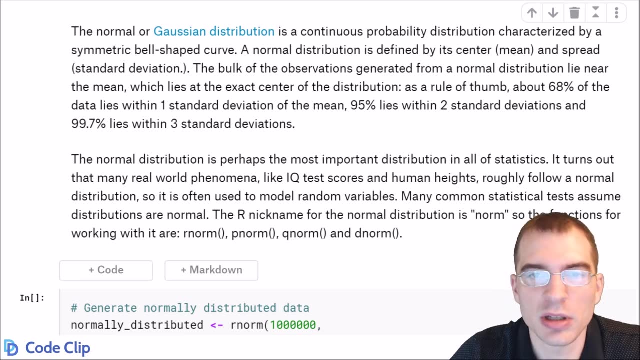 talk about something being within a certain number of standard deviations of the mean. these are good general numbers to remember because it'll give you some idea of the rarity of what they're talking about. Now. the normal distribution is perhaps the most important distribution in all. 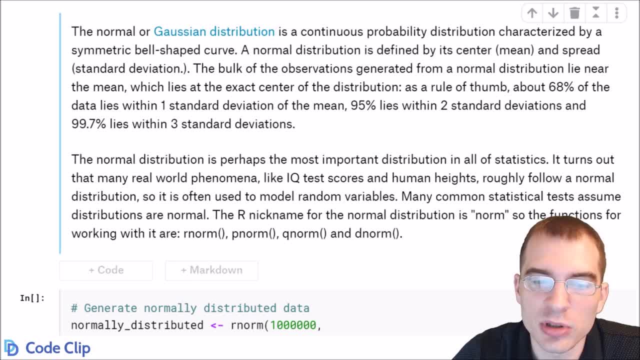 of statistics because, as it turns out, many real-world phenomenon like IQ test scores, human heights and other things that just naturally occur in the real world, follow a normal distribution. So, as a result, it is often used to model random variables and many common statistical tests and 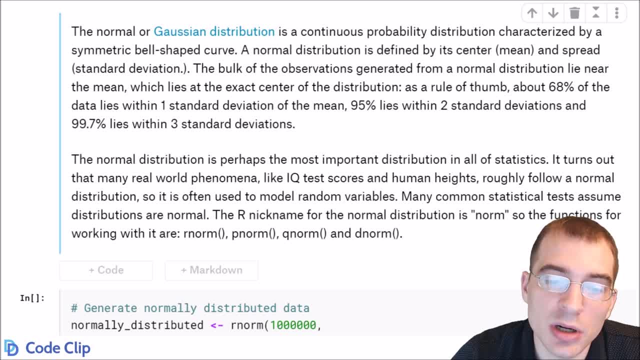 operations make the assumption that the normal distribution is the same as the normal distribution. Now, in R the nickname for the normal distribution is norm, so the functions you can use with it are rnorm, pnorm, qnorm and dnorm. You just take those prefixes we learned about earlier and 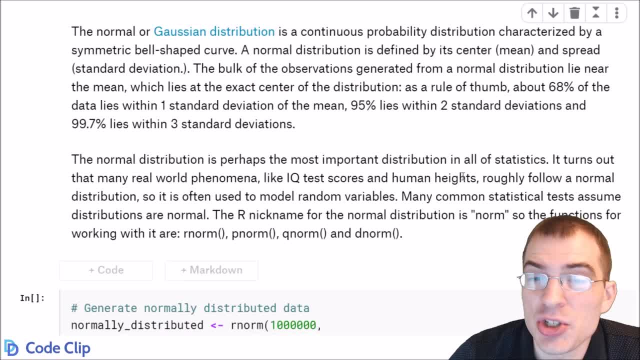 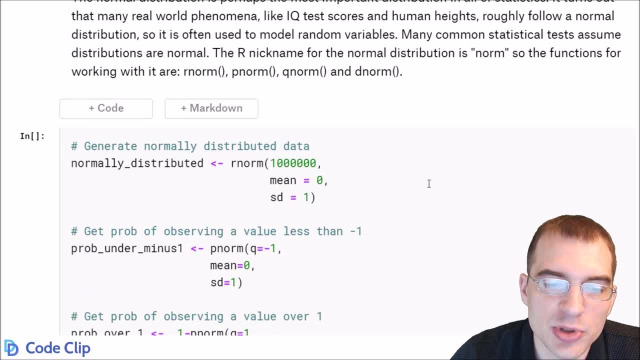 slap them onto the front of the name of the distribution. Let's generate some random data from a normal distribution using rnorm and then plot it to get a sense of what the normal distribution looks like. So this is a density plot of the normal data that we generated. 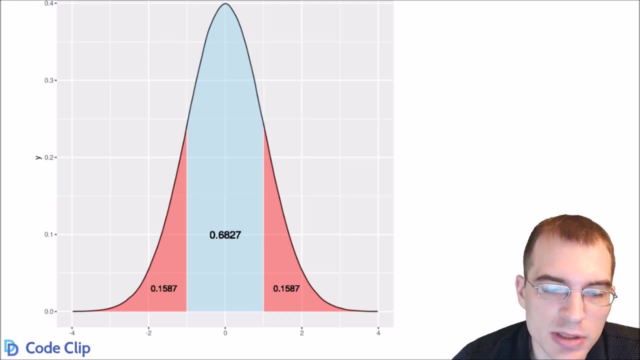 as you can see, most of the data lies within one standard deviation of the mean, and it also shows that values that are far away from the mean, which is at zero, perhaps at three or even four standard deviations, are extremely rare, because there's hardly any density under the curve here. 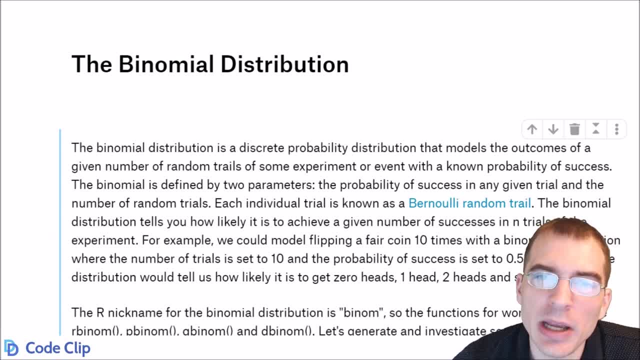 Next we'll go over the binomial distribution Now. the binomial distribution is a discrete probability distribution that models the outcome of a given number of Bernoulli random trials. So essentially it models the outcome of a given number of coin flips where the coin has. 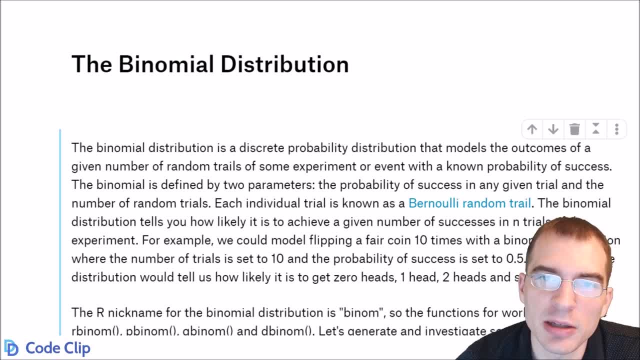 some underlying probability of success. p- The binomial distribution tells you how likely it is to get a given number of successes flipping the coin with a certain number of trials. For example, we could model flipping a fair coin 10 times with a binomial distribution where the number of trials 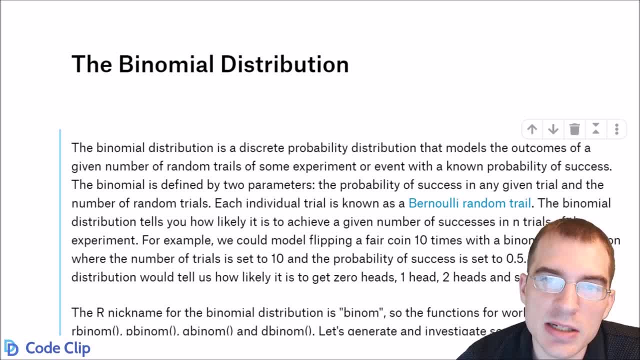 n is set to 10, and the probability of success for each of the independent Bernoulli random trials is set to 0.5. And the distribution would then tell us how likely it is to get 0 heads, 1 head, 2 heads, etc. all the way up to 10 heads. 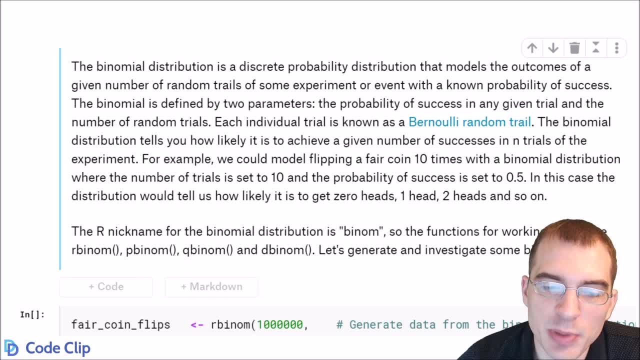 The nickname of the binomial distribution in R is binom, so we can use all of the prefixes we learned earlier with that: R-binom, p-binom, q-binom and d-binom. Let's use R-binom to generate. 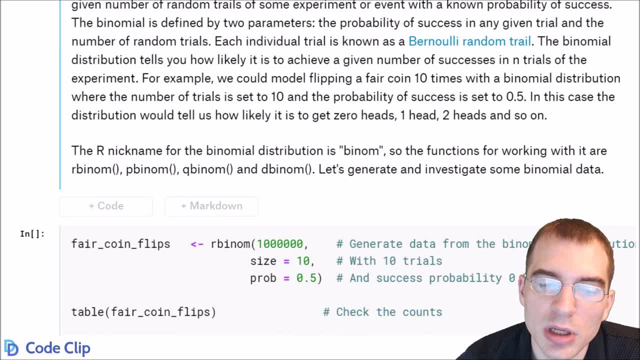 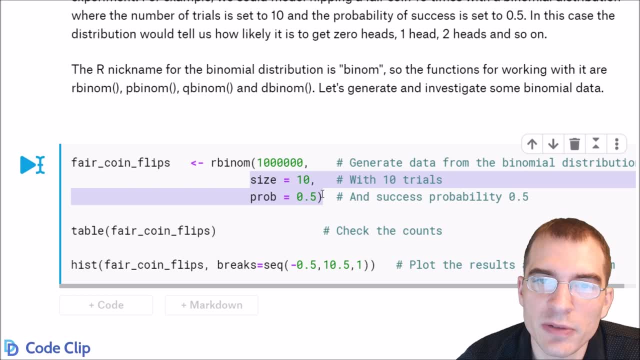 some random data from a binomial distribution. We'll have 10 trials with a probability of 0.5, so we're essentially modeling the distribution of flipping a fair coin 10 times. So we'll run this and create a histogram of the result to get an 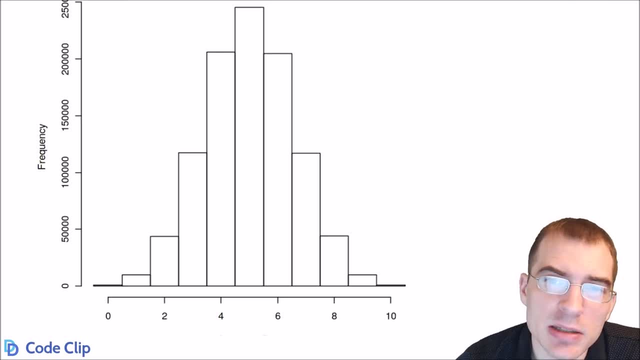 idea of what the distribution looks like. As you might expect intuitively, if you were to flip a fair coin 10 times, the most likely outcome is that you'd get 5 successes or 5 heads, and it's very unlikely that you'd get, say, all heads, which would be 10,. 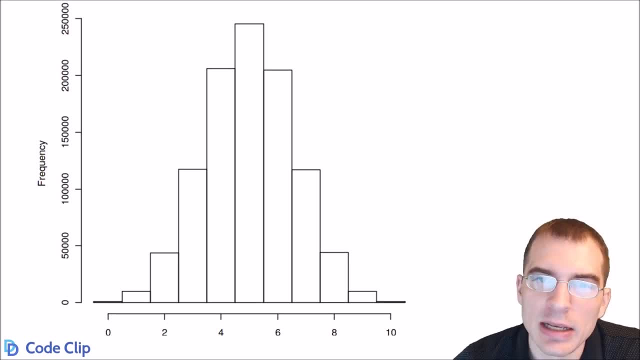 successes or 0 heads, which would mean you got all tails. In this case the distribution in the histogram is symmetric because we had equal chances of getting either result. but if we changed the value of p, which is the probability of getting a success on? 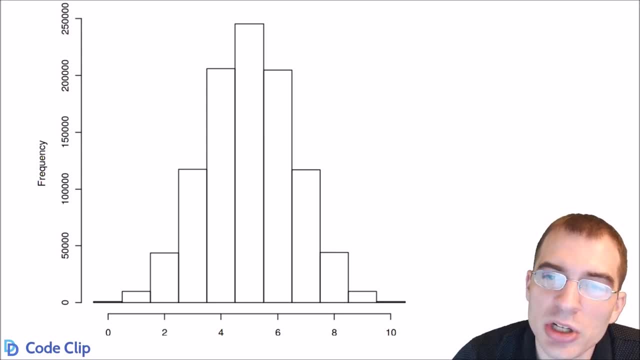 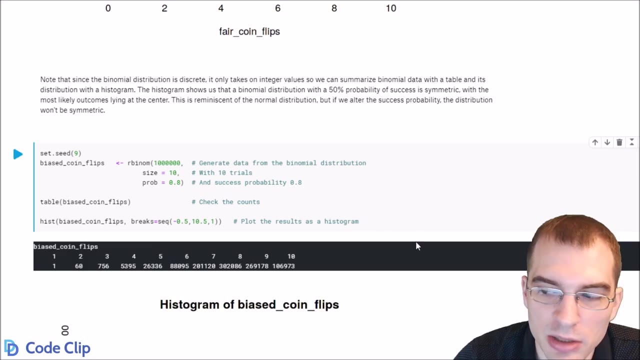 any given trial. this would not be symmetric anymore. So let's generate some new data, but let's use a biased coin where the probability of success is actually 80% instead of 50% and see how it changes this distribution. So I'm just going to generate that extra data and run another histogram and, as you can see, 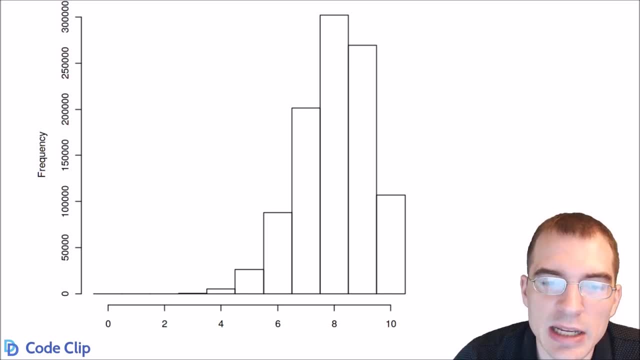 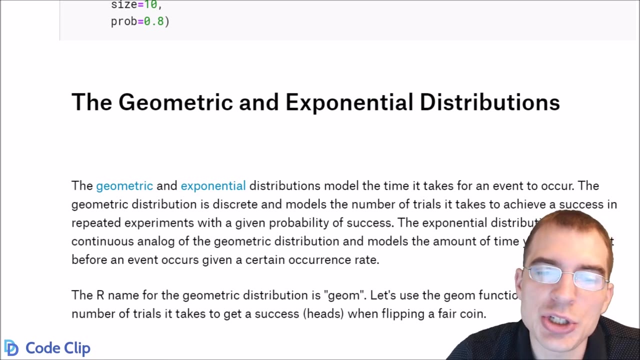 this time, when the probability of success is 80%, the most common outcome is that you get 8 heads out of 10 flips. But now getting 10 heads is actually quite common and the chances of getting no heads at all is extremely low. Next we'll go over the geometric and exponential distributions. 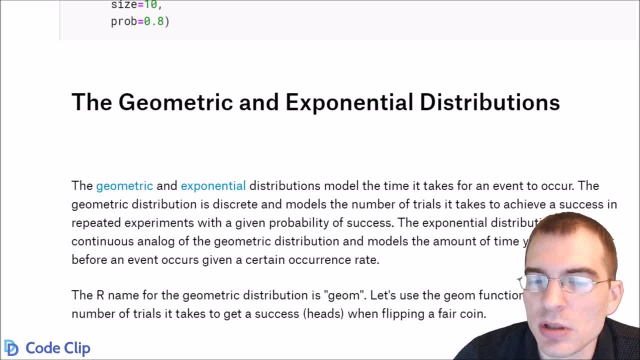 Now the geometric and exponential distributions model the time it takes for some event to occur. The geometric distribution is discrete and models the number of trials it takes to achieve a success on some repeated experiment, with some given probability of success. For instance, you could model the amount of trials it 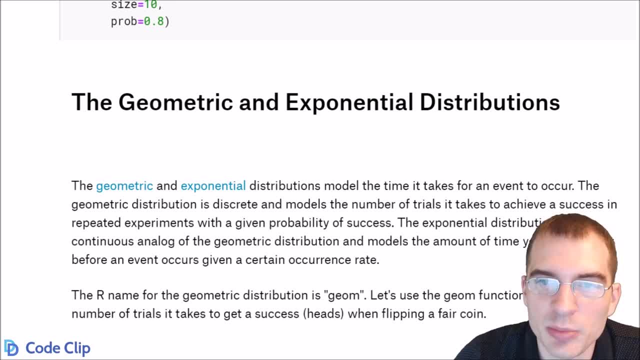 would take to flip heads on a fair coin if you repeatedly flip it. And the exponential distribution is essentially the continuous rate of success. That means, for example, if you were to continuous analog of the geometric distribution that models the amount of time it would take for some event to occur, even some. 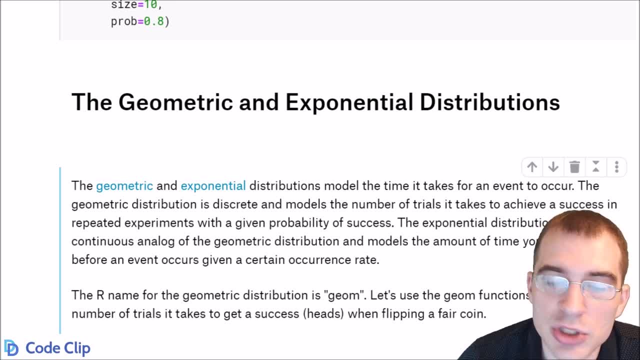 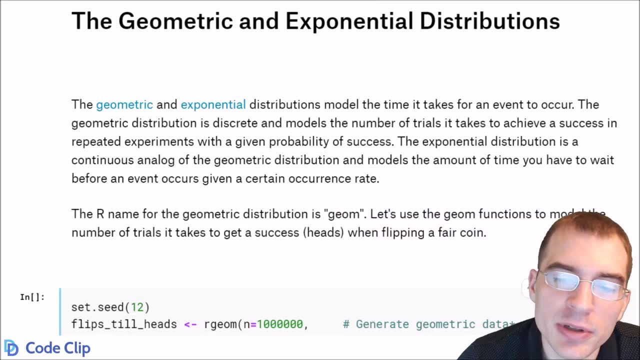 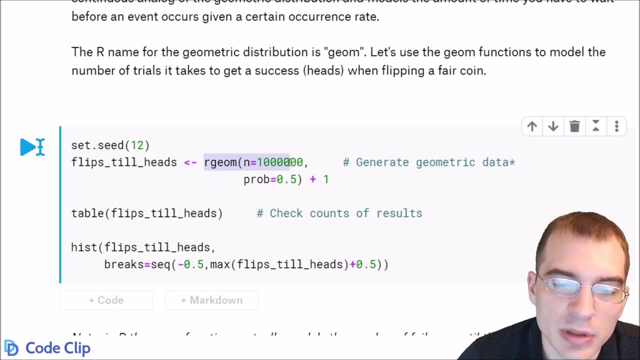 Specified occurrence rate, the. our name for the geometric distribution is geom, so let's use that to generate some random geometric data and Model the number of trials it takes to get a success when flipping a fair coin. So to do that, we're going to use our geom and then we're going to set the probability to zero, point five. 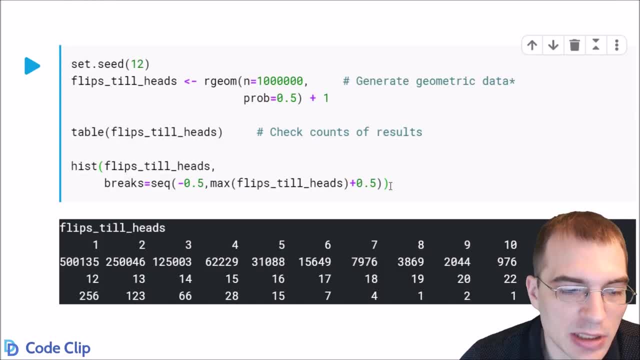 So it's a fair coin. so let's run that. and we see that out of a million trials, about half of the time- 500,000- it only takes one flip to get a heads. that makes sense. then 25% of the time, essentially it takes two flips. 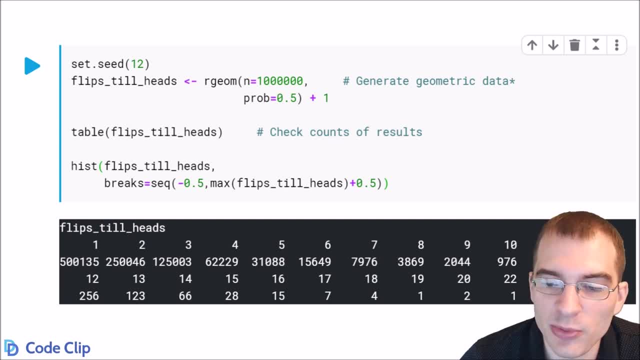 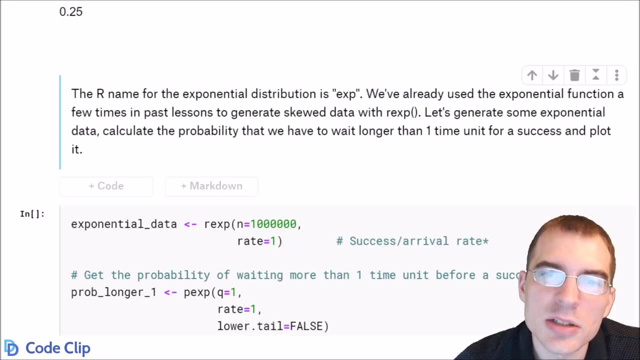 Etc. So we actually had one time where it took 23 flips before we got a heads, But that is extremely unlikely because that only happened one out of a million trials. So let's do the same thing for the exponential function in our the name for the. 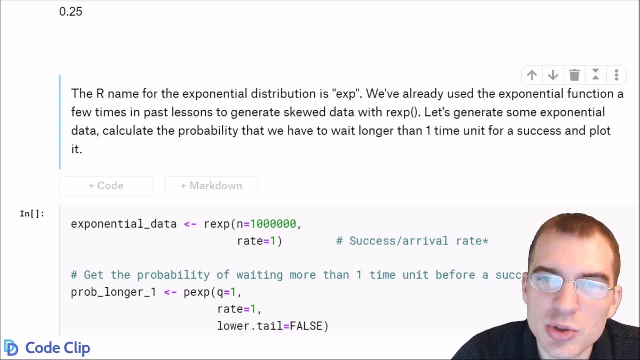 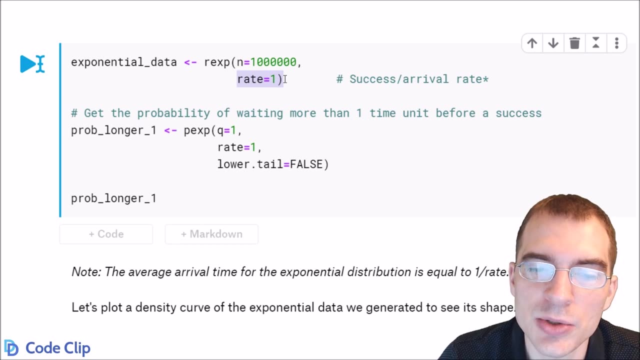 Exponential distribution is X. we actually use this in past lessons to generate some skewed data. Let's use it again to generate some random numbers. here We're going to use our X to do that, and the rate indicates how often a success or arrival occurs Per unit of time. so here we're setting the rate equal to one, which means we're expecting one success or arrival. 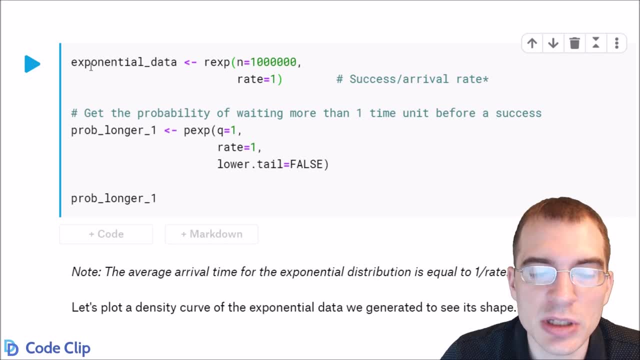 Per unit of time, which means, for instance, if we were using this to try to model, Say, arrivals of patients at a hospital, and we'd have one patient arriving per hour, Just going to run this, to generate the data, and then this next bit is going to make a plot. 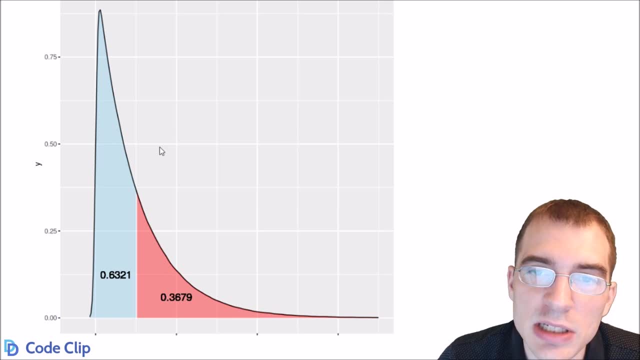 looking at the distribution of the data, as you can see, with an average arrival time of one, most of the time a Success occurs in less than one unit of time. You can see that 63% of the time, it takes less than one for an arrival to occur occasionally in this long tail. 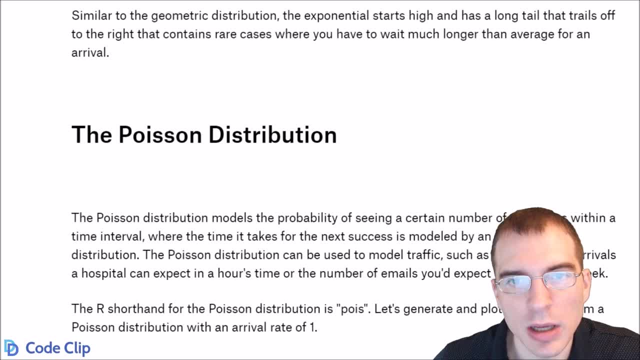 It takes much longer for a success to occur. and finally, we are going to discuss the Poisson distribution. the Poisson distribution Models the probability of seeing a certain number of successes within a certain time interval, Where the time it takes for the next success to occur is modeled by an exponential distribution. 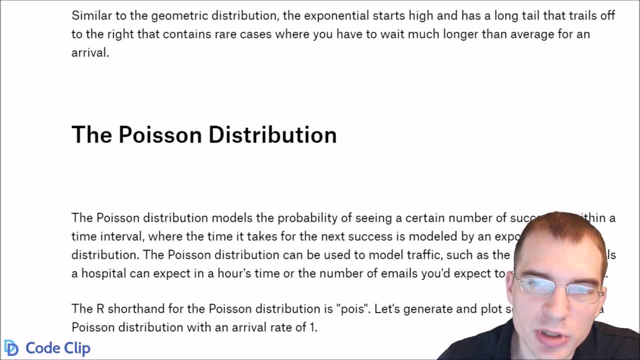 So when we were looking at the exponential distribution, We were talking about, say, how long it takes for the next patient to arrive at a hospital if the average arrival time It was an hour. the Poisson distribution, on the other hand, would tell us things like how often 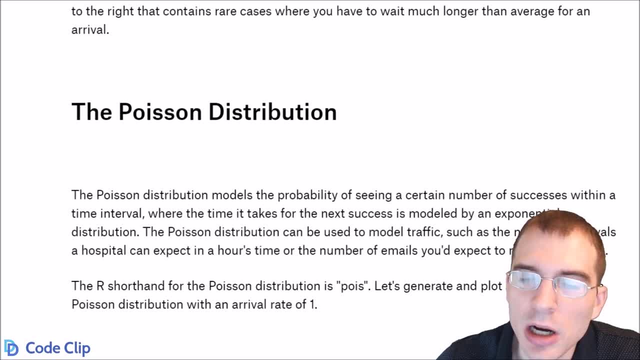 We would have zero arrivals during the first hour. How often would we have only one patient arriving within the first hour? How often would we have, say, 10 patients? and having an unexpected busy hour Are the nickname for the Poisson distribution is poise. 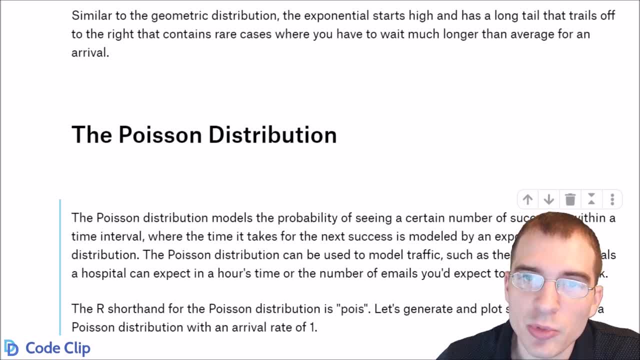 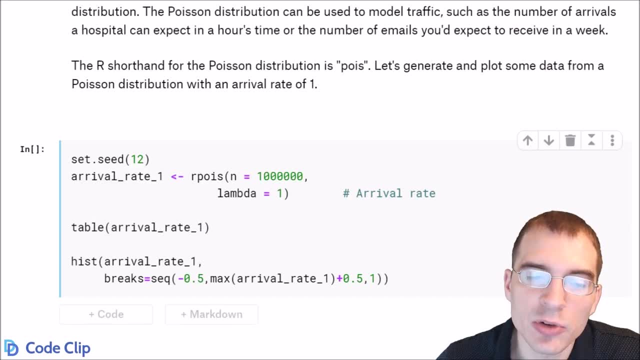 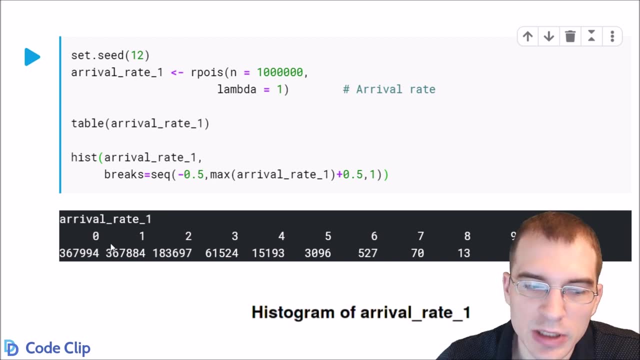 So let's use that with our, our prefix, to generate some random Poisson distributed data and get a sense of what Distribution can look like. we'll be using an arrival rate or lambda of one. The table here shows that with an arrival rate of one, more often than not, 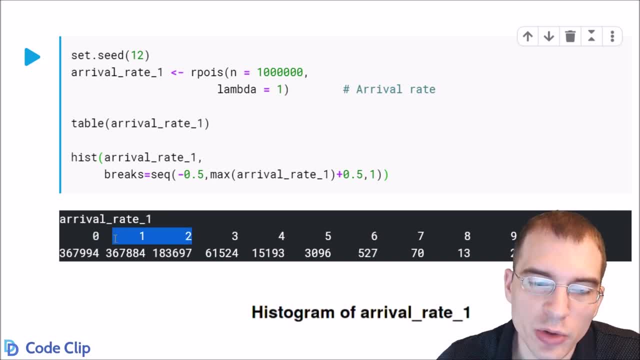 We're only going to see zero, one or two arrivals within Given time period, but sometimes- in rare cases- you do get seven, eight, even nine arrivals. so while it's not likely, businesses would still have to account for the possibility of getting a rush of people that's more than expected, and if 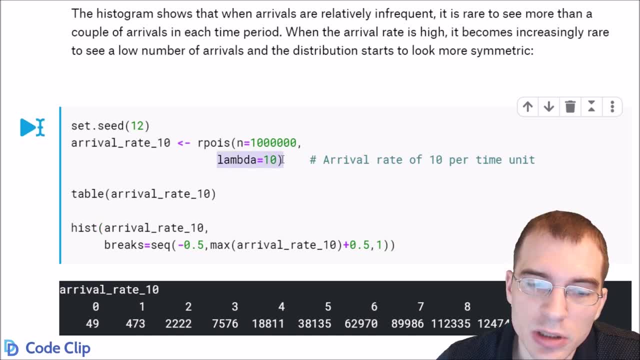 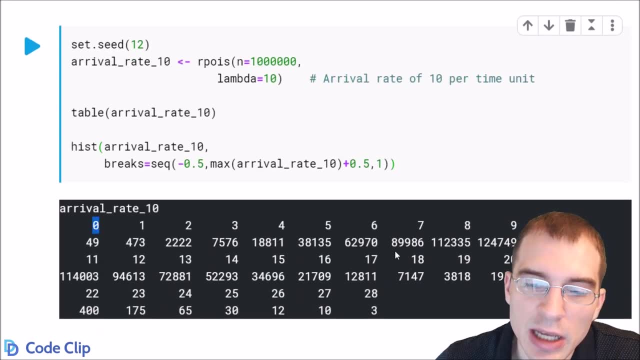 We were to set a higher arrival rate, so we'll do a arrival rate- or lambda- of ten this time. It's actually not very likely to have zero arrivals anymore, But we're far more likely to have many arrivals if we plot a histogram of the distribution.